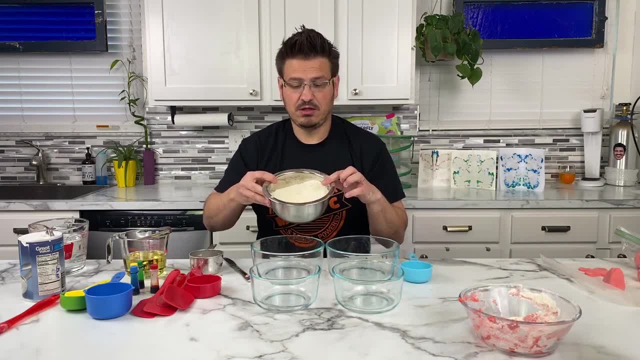 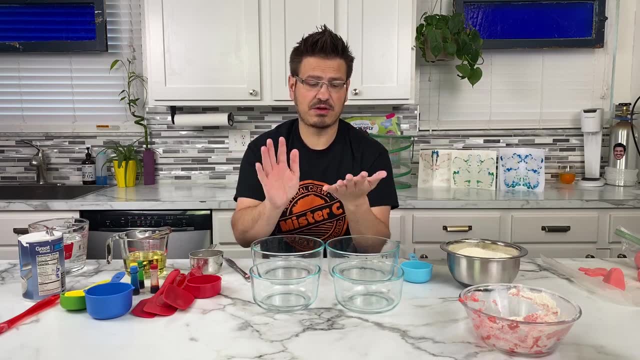 always add color afterwards, like you can make a big batch with the flour and the salt and then split it up and do the food coloring. but look at my hands. they're relatively not red. i mean, there's a little bit of red too, but if i go wash my hands they'll come right off. so i like to do it. i like. 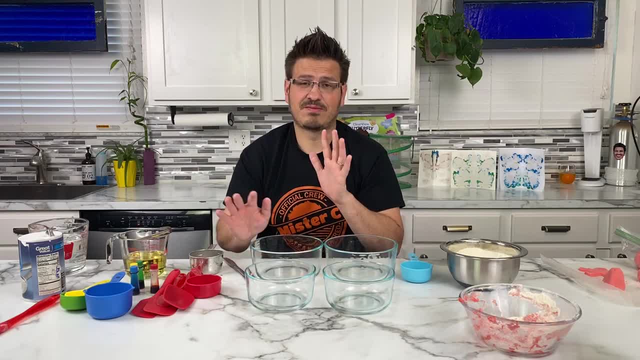 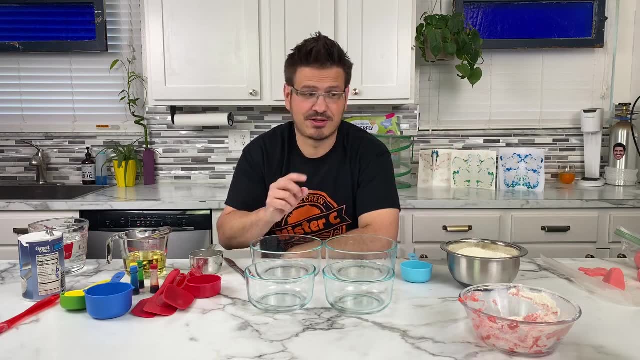 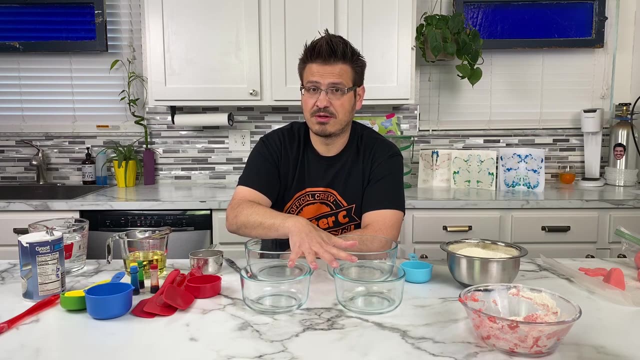 to add food coloring to the water beforehand because it really minimizes the mess. but it's just the mess, it's food coloring. it should come off. keyword should: all right. so we have two cups flour total. so now we have four bowls. we're gonna do a half a cup in each of our bowls all. 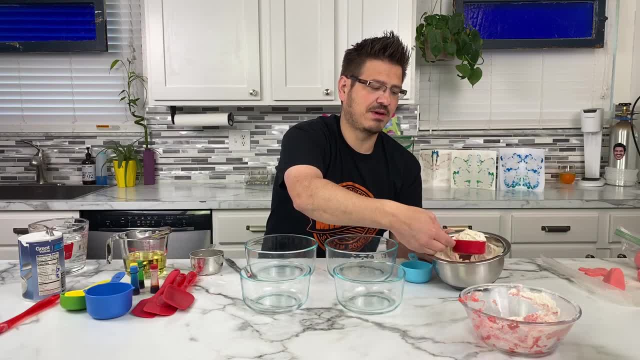 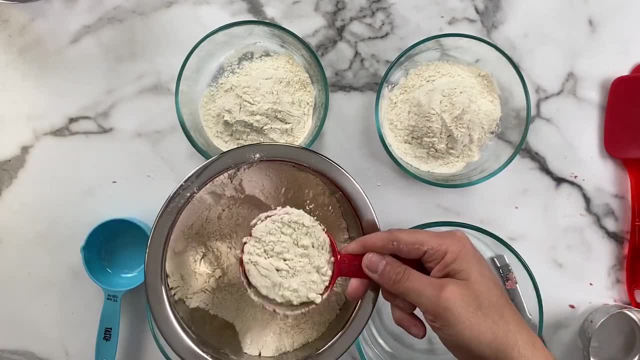 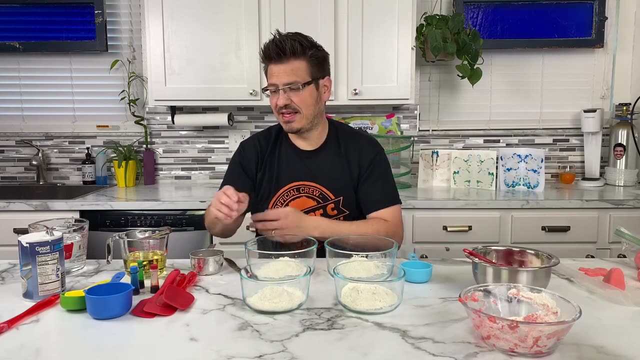 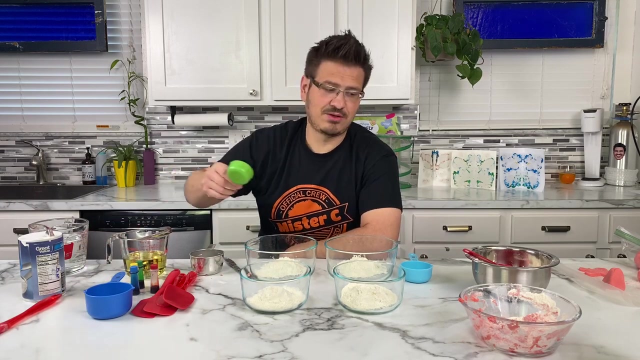 right, half a cup of flour in each of our bowls. so now we're using, busting out those math skills: boom, half a cup, boom, half a cup, all right. and then what we have is a half a cup of oil total. so now we get into understanding math a little bit. so half a cup of oil would have been mixed. 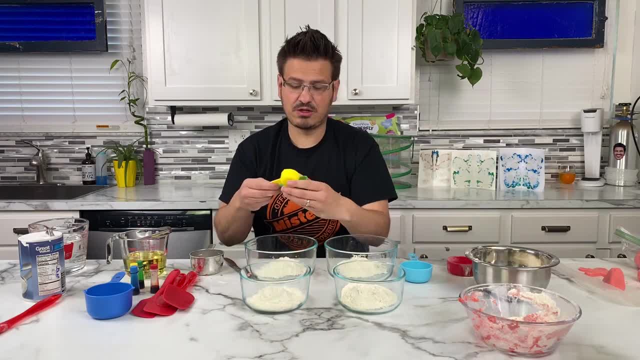 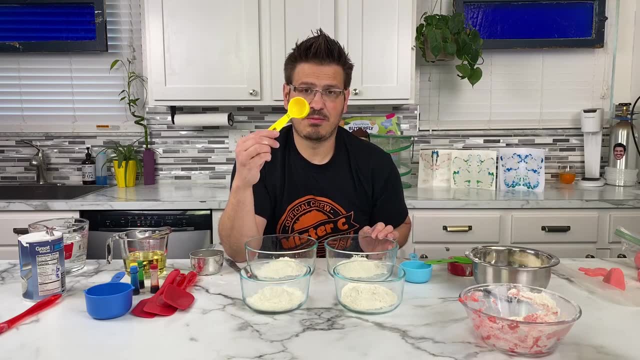 to all of this. if we break that in half, we're only doing two. you use a quarter cup in each of them, but since we're doing four, we take the half cup and we use an eighth of a cup, because four eighths is actually one half. all right, so we're gonna add half a cup of oil to each of these. 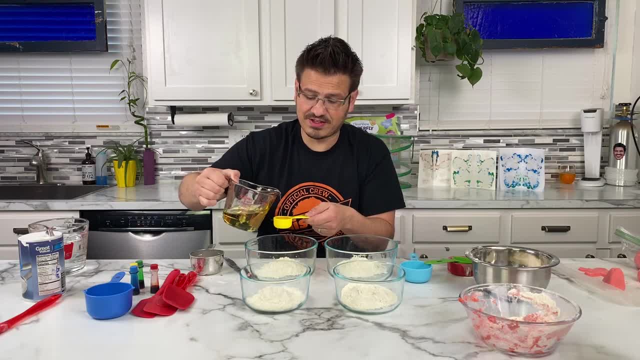 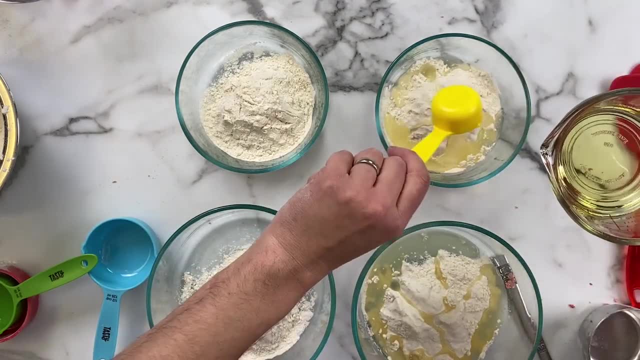 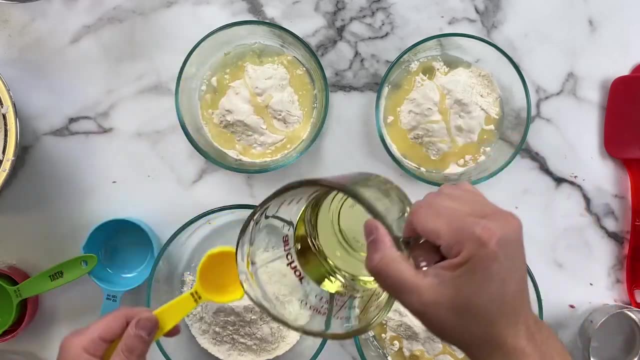 cups. all right, so we're gonna add half a cup of oil to each of these bowls and we're gonna add half a cup of flour. all right, so that's our half a cup of oil, and just so i've said it. i have never done this recipe, so this is a true experiment. 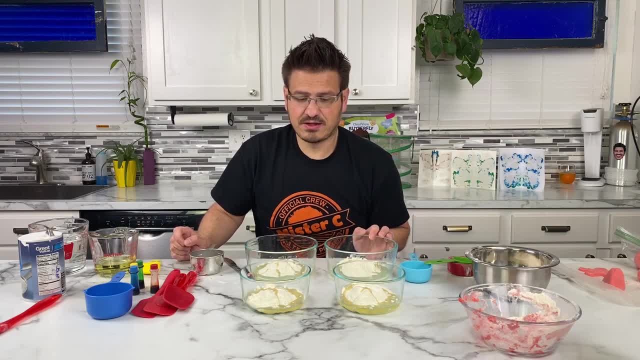 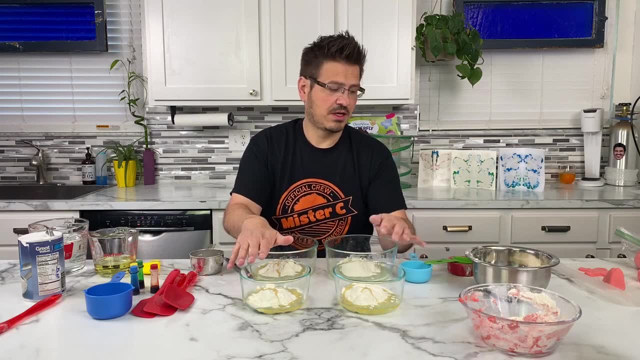 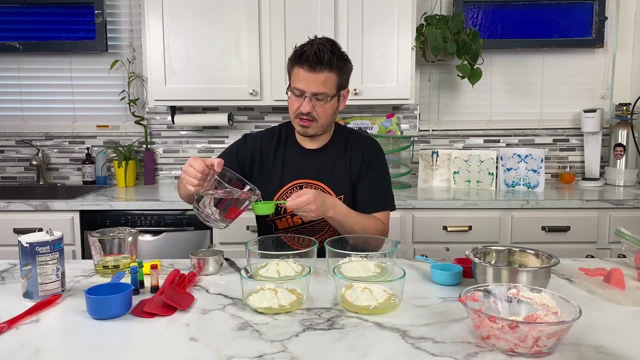 i found it online. i found other things online that work and don't work sometimes, so we're just going. so if we had two, each one would get a half a cup, but since we have four, each one gets a quarter cup of water, so we did red over there, but i think we're going to do another red. 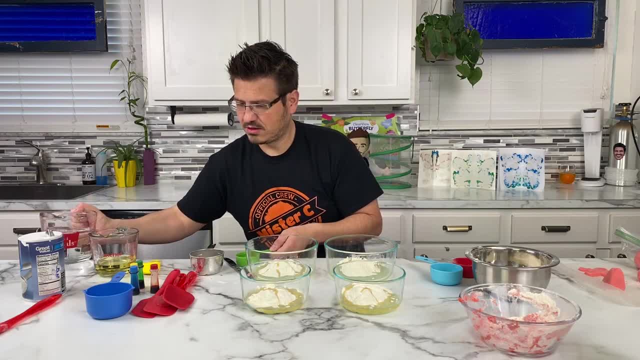 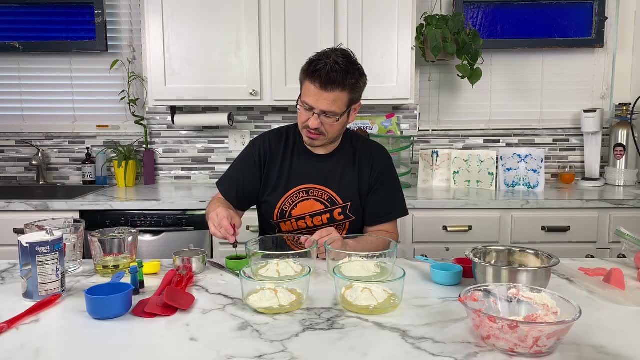 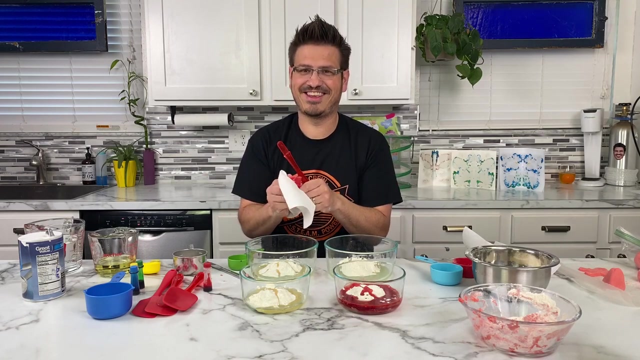 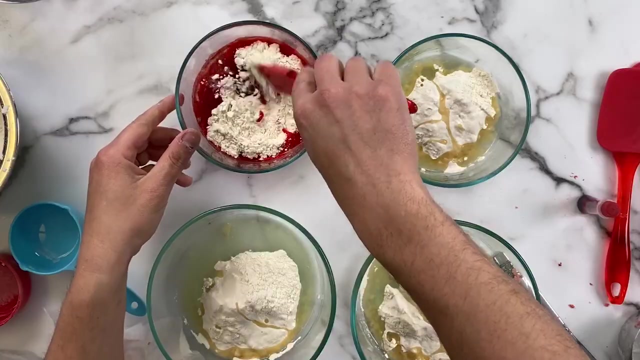 just so that we have a comparison, curious what it's going to do with the oil. so i'm gonna do lots of red here, really, really red. i'm gonna put that one into that. well, that wasn't good. i just ripped our little spatula. sorry, missus c. another one bites the dust, all right, so we're gonna mix that up. 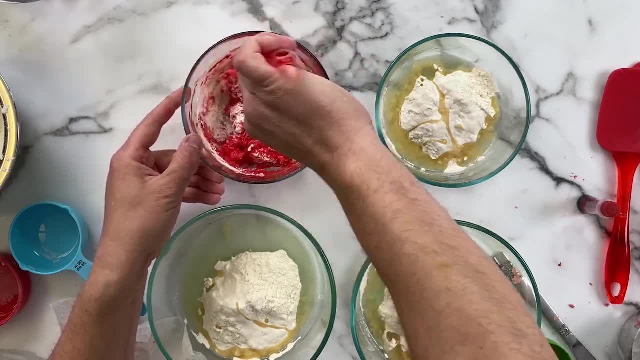 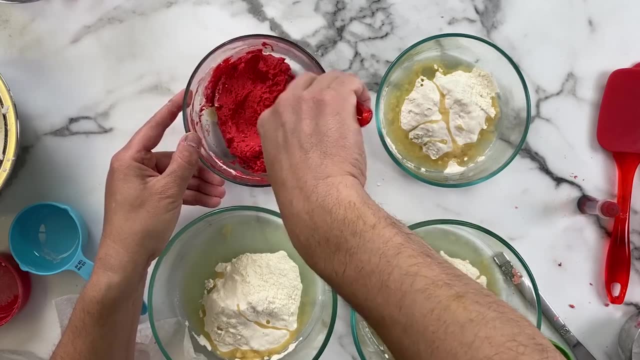 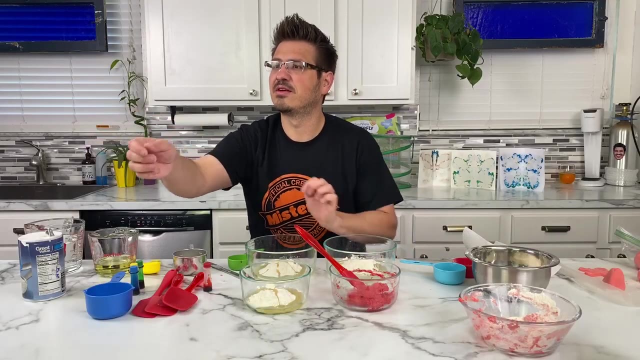 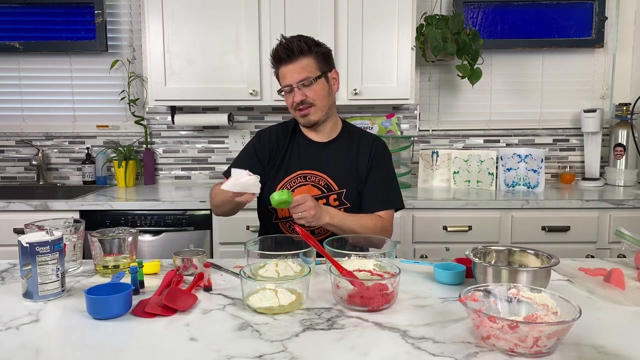 oh, the texture is totally different. you all right, i kind of like it, though. yeah, i'll use that one, we'll use, we'll use a little blue and we're gonna do blue, all right, so i'm gonna get the red out of here, so we don't. 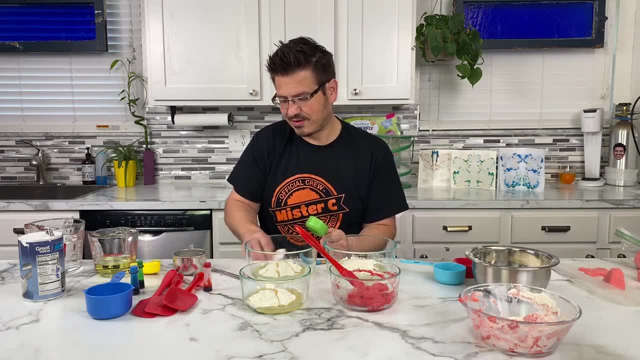 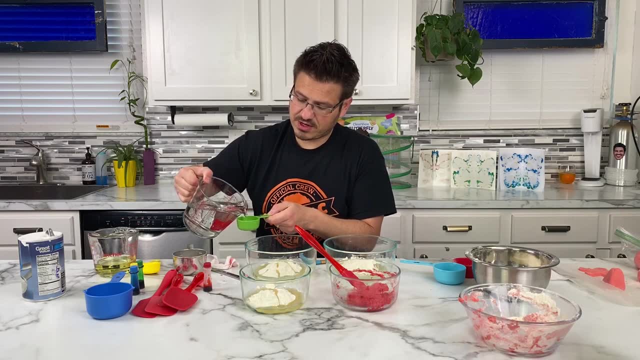 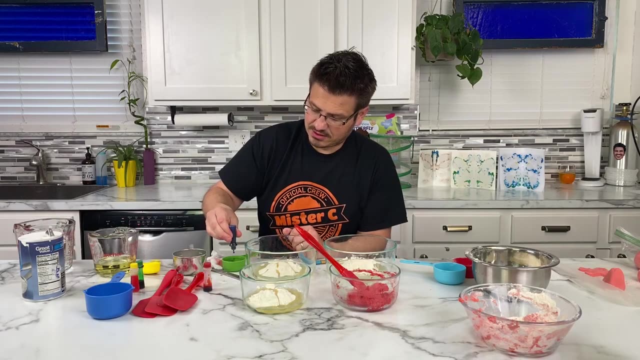 mix in the red with our blue, otherwise we would get purple. all right, so we do our quarter cup of water. make sure i have this right and we're gonna do blue, mr c's favorite color this time. i'm gonna stir it up just ever so slightly. 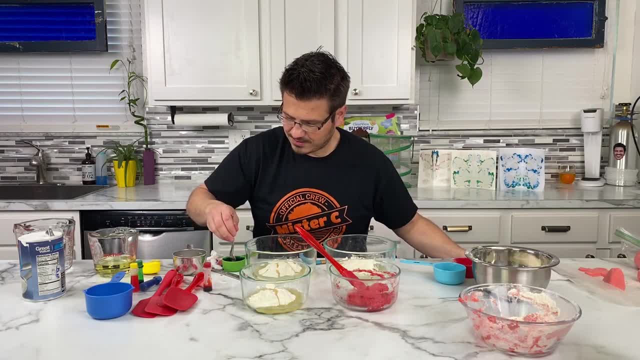 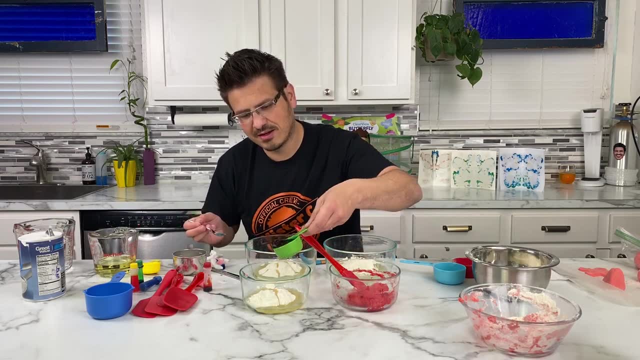 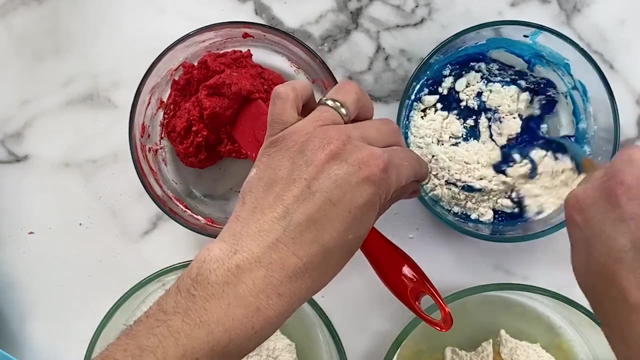 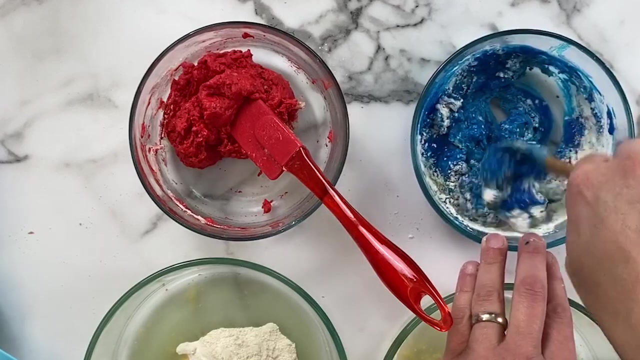 so it doesn't get stuck, so i don't lose the blue. all right, left-handed, perfect. all right, i can use my little blue. these colors. it's really vibrant, isn't it? compared to the other one. i also added a lot more food coloring, but i think it has something to do with the oil. 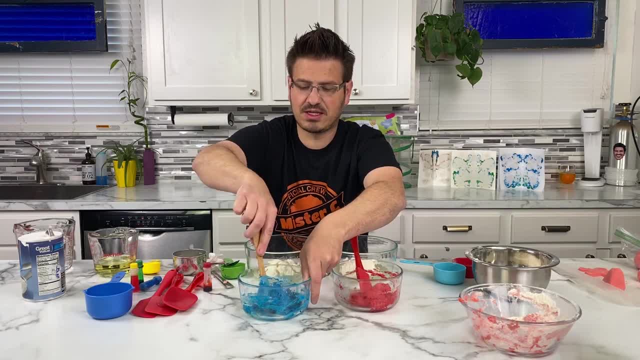 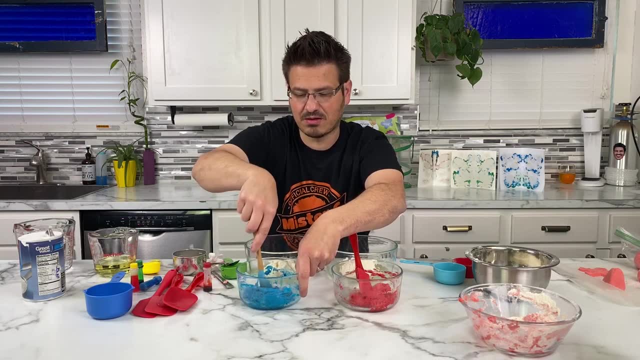 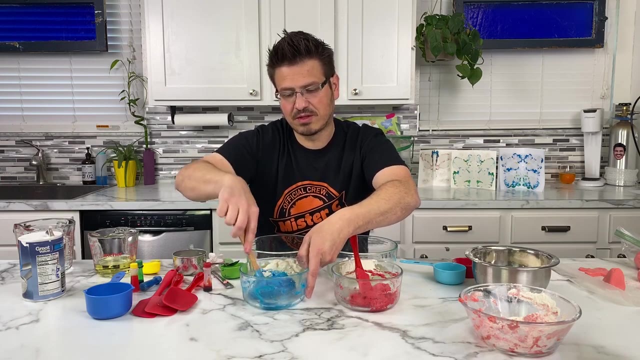 and i think we're gonna have to add a little bit of flour to this in a second, because it's really feels sticky. i haven't put my hand in yet because i'm going to set all these up and get them all going. oh that's, that's really cool. that feels really awesome. 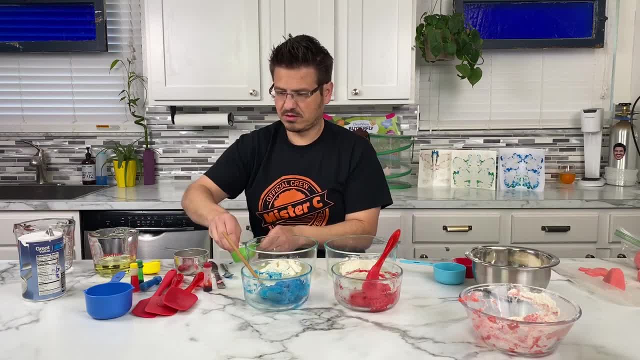 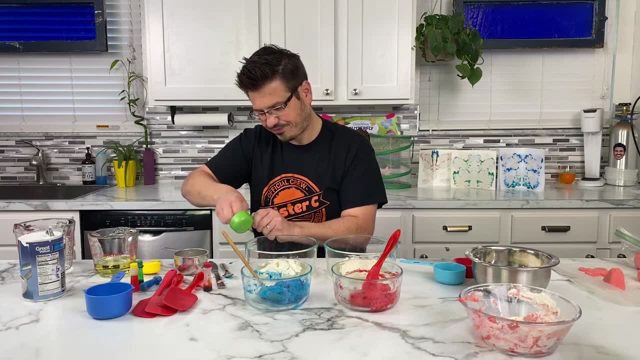 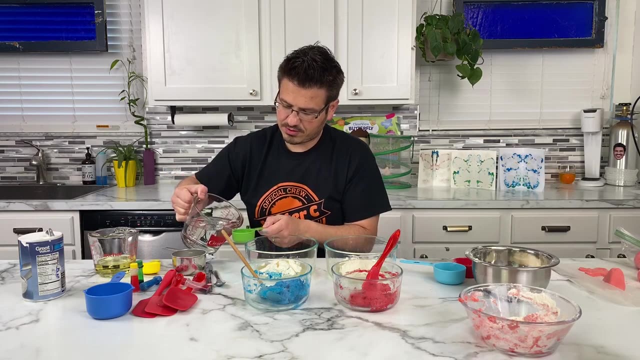 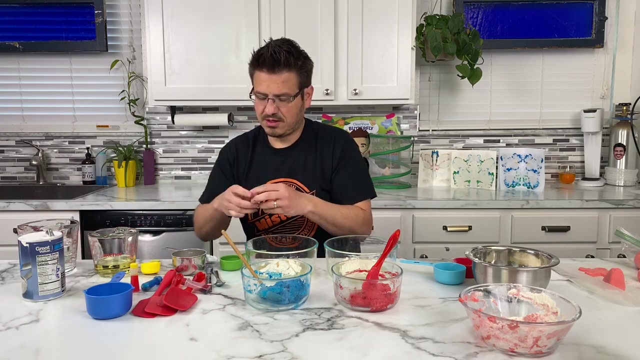 all right. so now we're going to do our. we'll do green. we'll just go with the colors, the fruit coloring colors, unless there's a crazy color someone wants me to try to make. all right, here we go. quarter cup: our measuring spoon measuring cup is green. do you want to put it in a bigger cup so you have room to mix. 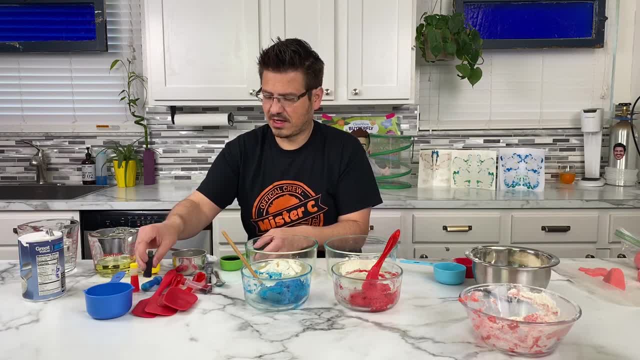 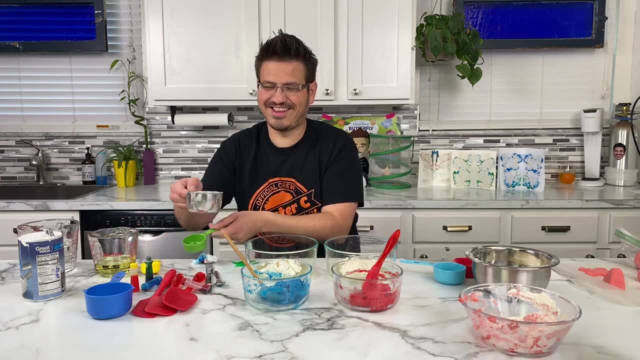 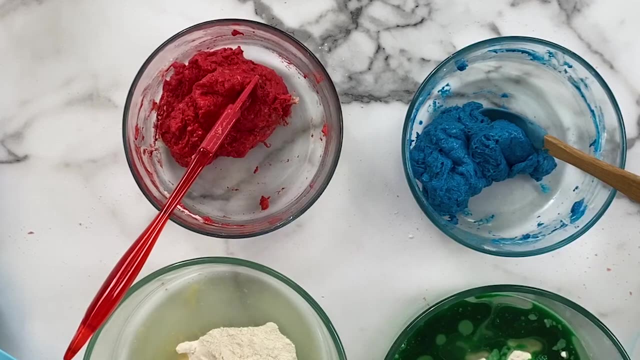 i'll do that on the next one. i guess i could just pour it in there. right, there we go. oh well, if we're not making a mess, we're not doing something right. we're not making a mess, we're not doing something right. and our green, all these colors are just 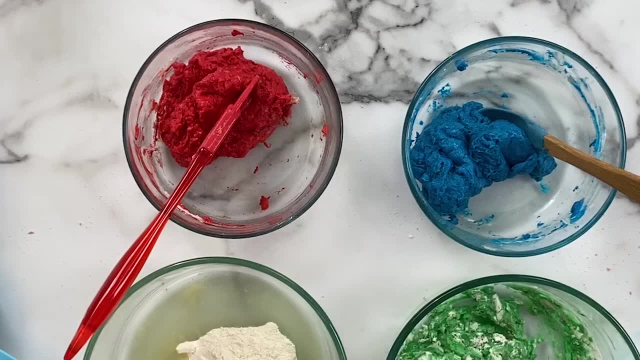 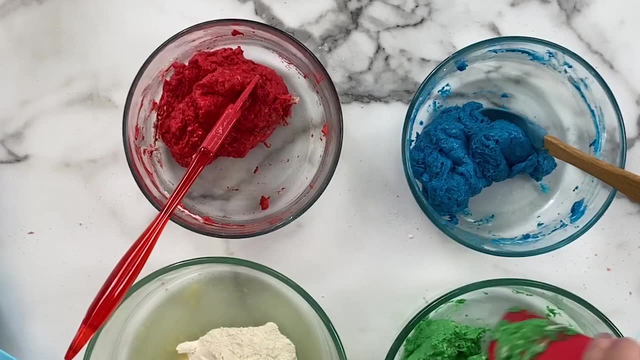 fantastic. our friend james said: make purple, purple. and our friend dave said: make black. but i think we have to mix them all together. yeah, i don't know if i have black. would be cool to try to make, i'm just afraid it would get really, really messy. let's try purple. let's try purple. 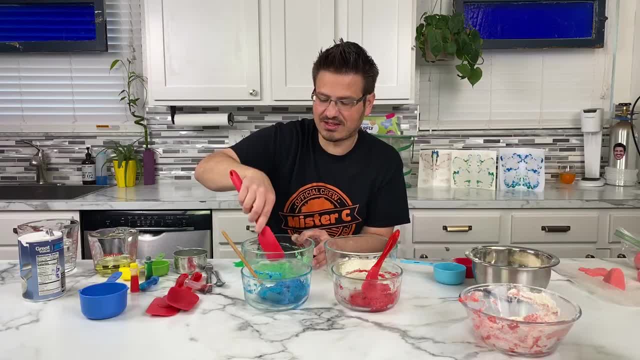 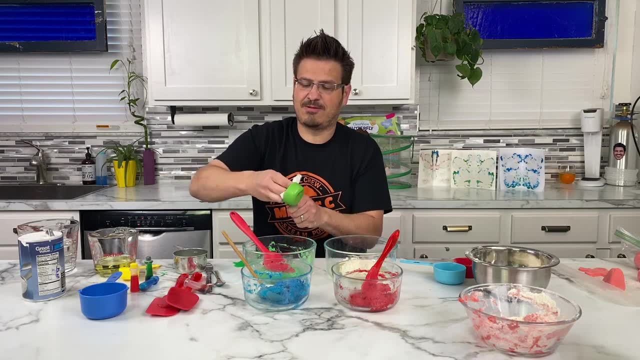 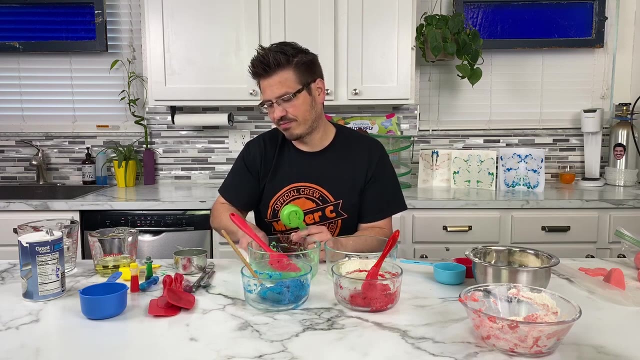 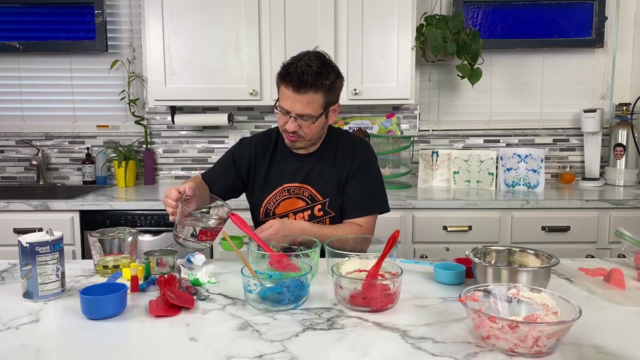 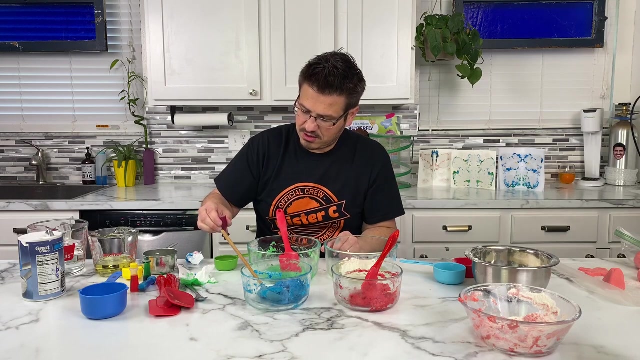 oh it's, it's really, it's kind of slimy. i'm just gonna throw the rest of that in there. all right, i'm making a little bit of mess, all right, that's all right, that's okay. we're doing science and math today. all right, to make purple we need red. or in german we say: 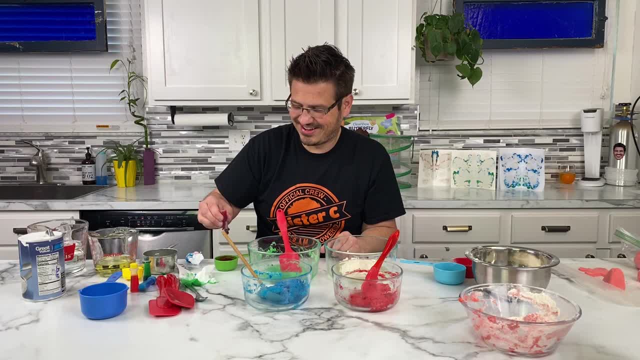 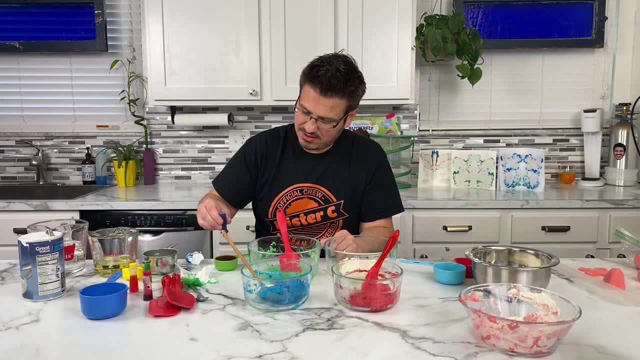 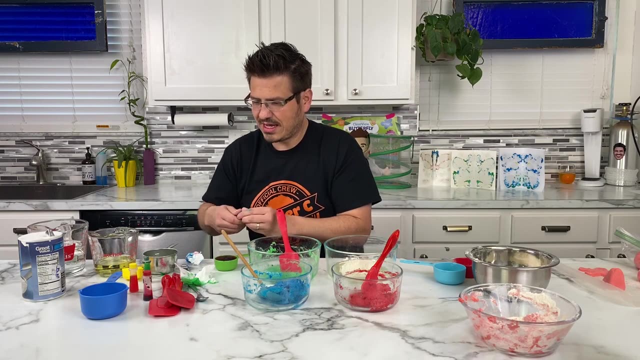 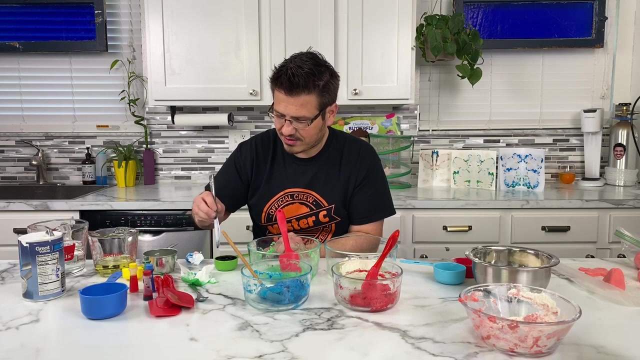 rock, say, rot did four drops there, Rot und Blau. Oh, I'm on the side of blue. Nein, All right, because I use the blue on this knife. I can stir this. Here we go, All right, I'm excited to see what this looks like. It's dark. 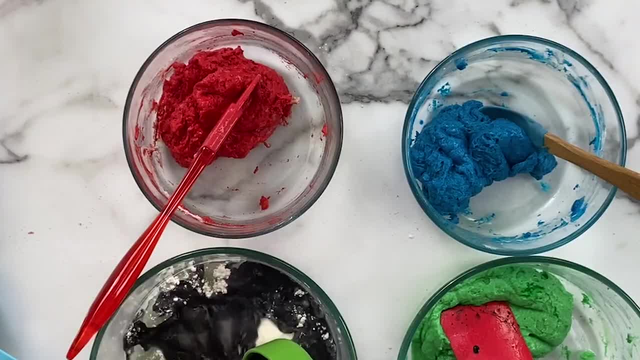 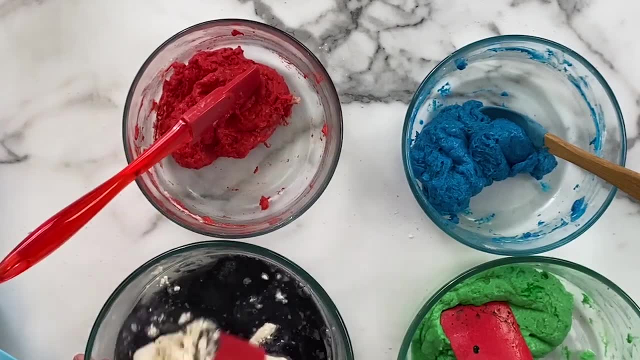 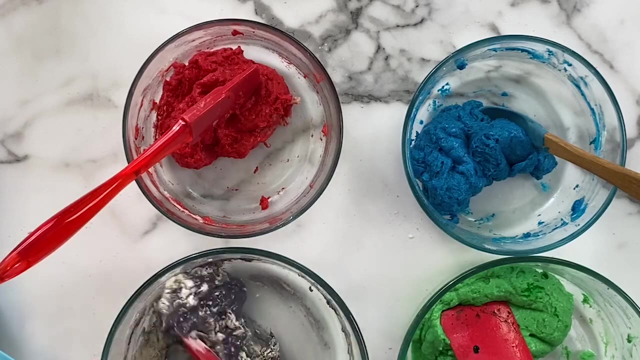 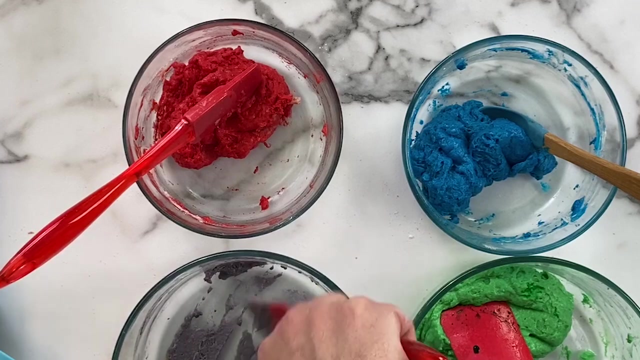 Look, Here we go. Oh, it's almost like black. Look how dark that is. Move that out of the way, All right, so we're going to bust these out here in a second. We're going to start with the green. 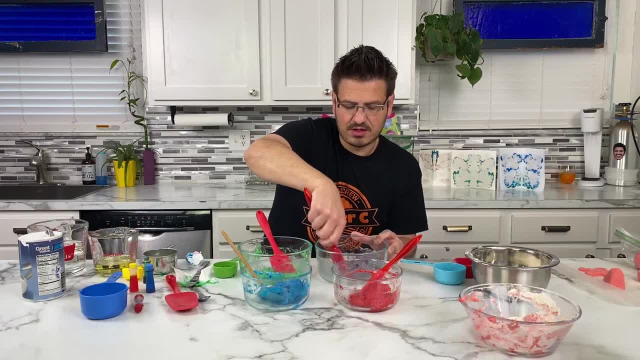 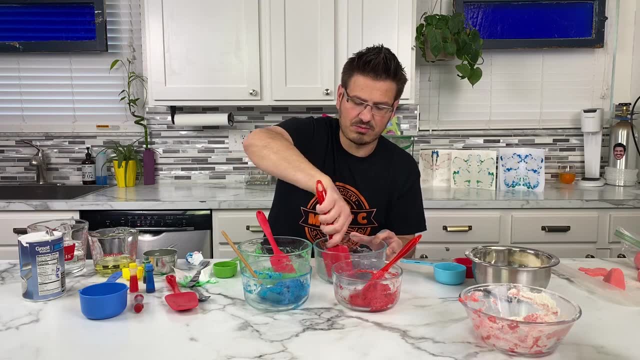 Now we'll start with the red, then we'll do the blue and we'll do the purple, because if we have some remnants of those colors on the table, they'll kind of mix together. It won't be too bad. I'm going to move these out of the way, just so we have a little bit. 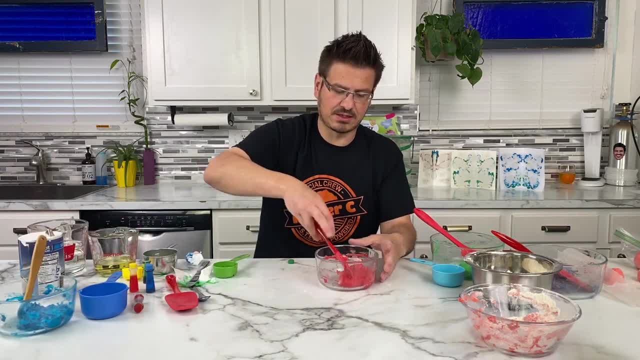 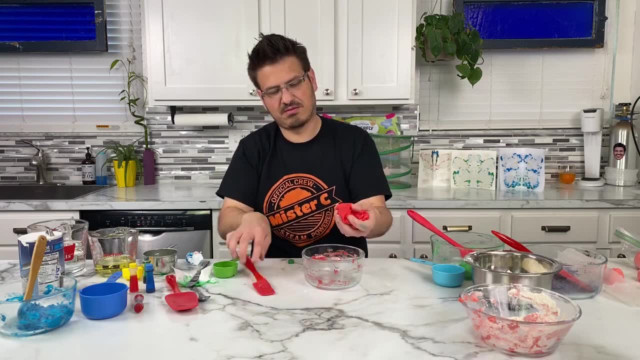 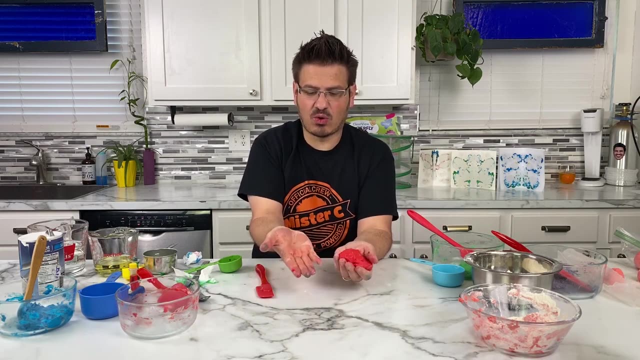 of space to work and knead. I need more space, All right, Oh, I didn't mix that very well down here. Here's where it gets. Oh, Oh, it looks sticky, but it's okay. It's oily, so it's a little oily. 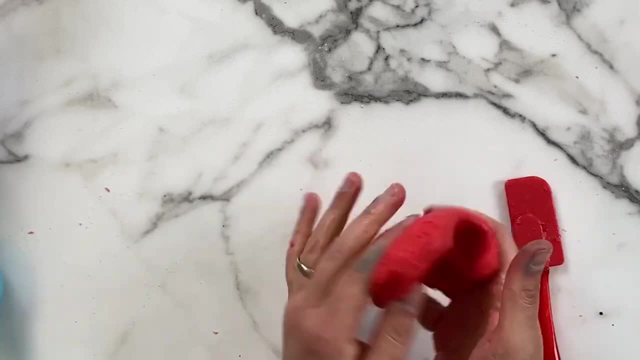 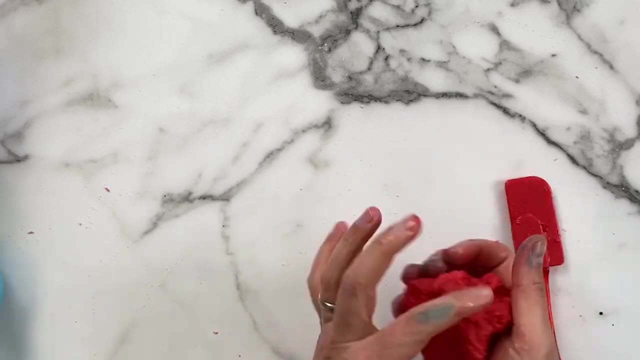 This might be an outside play-doh, then I think, yeah, I mean, this is definitely something you want to keep at the table. You do not want to take this out to the living room and get it on the couch or furniture. All right, I'm just going to sprinkle some. 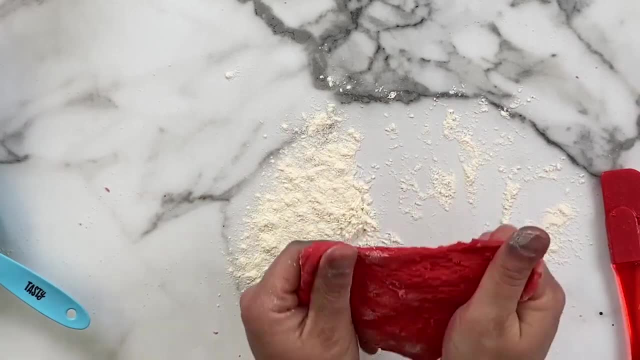 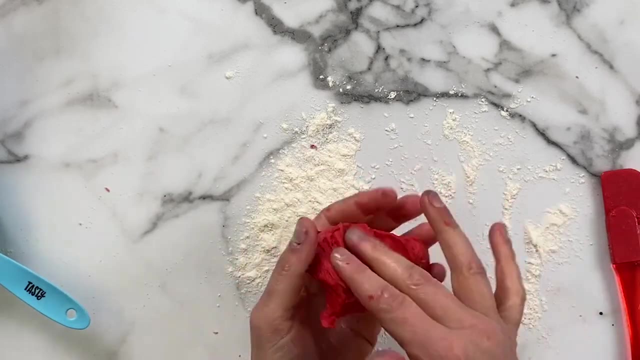 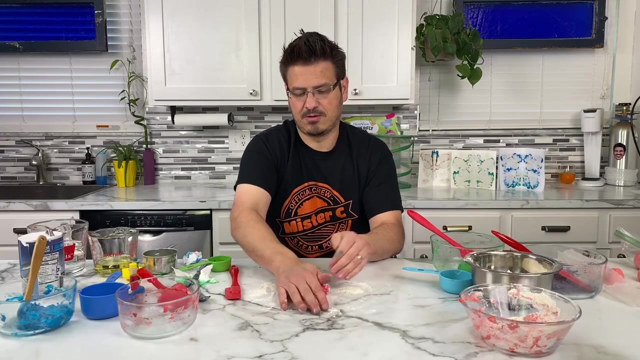 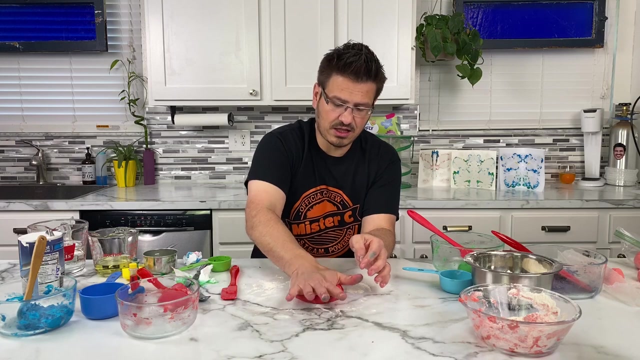 Yes, it needs just a little bit. Look at that. Okay, Out of the two, I like the texture of this one better, But it's a little greasy. And see, my hands are pretty much not changing colors. That's because I added the color beforehand. 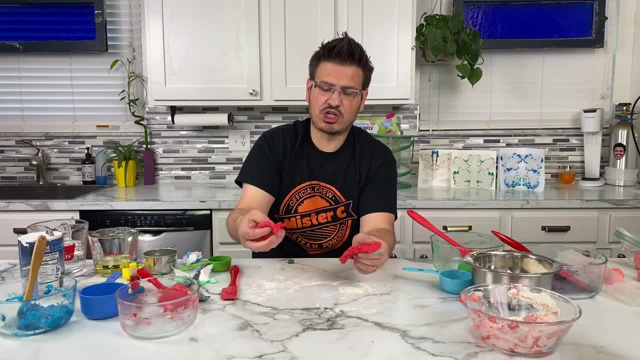 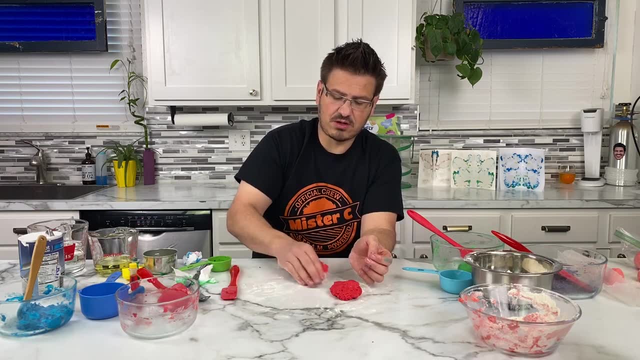 But my question is this: Will it hold a shape like the other one? Here's the test. Yeah, I think it's. It's harder to hold a shape. So the salt All right. so these are two different types of play-doh. 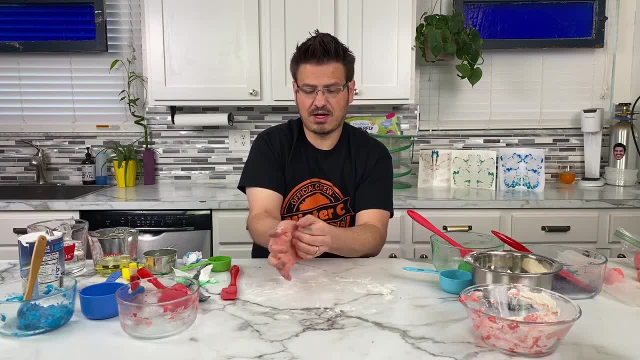 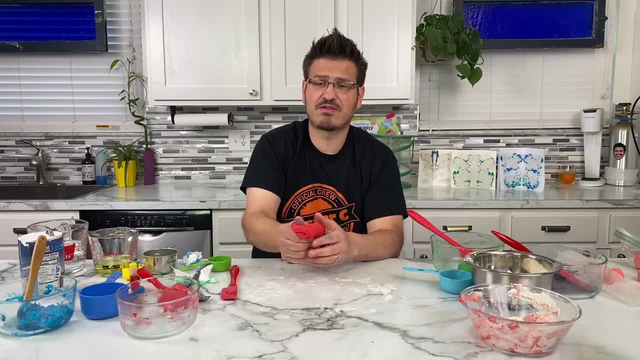 All right, let's get the other color going. All right, I'm happy with it. Oh, I like it. The texture is really cool. It's like slime- almost That's how it feels. It feels like slime without the stretchiness. It really does feel like slime. So there's. 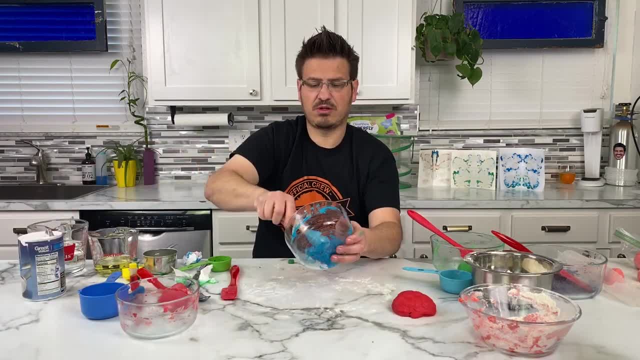 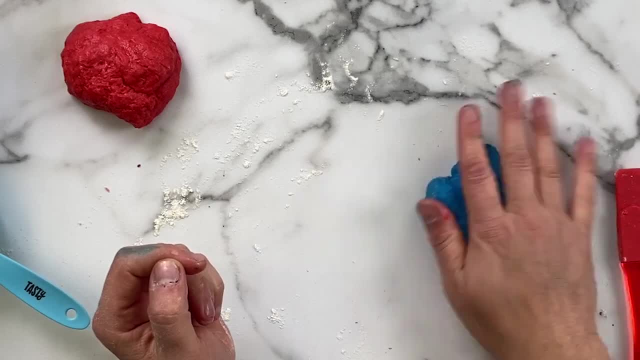 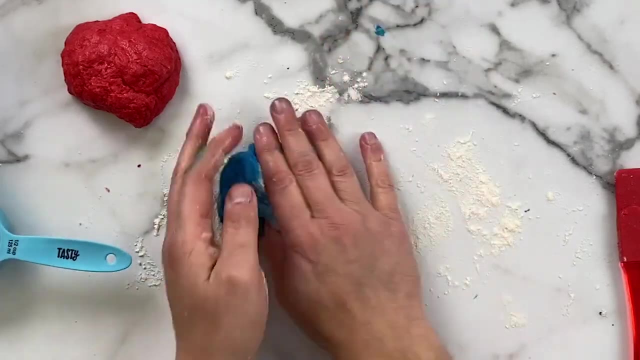 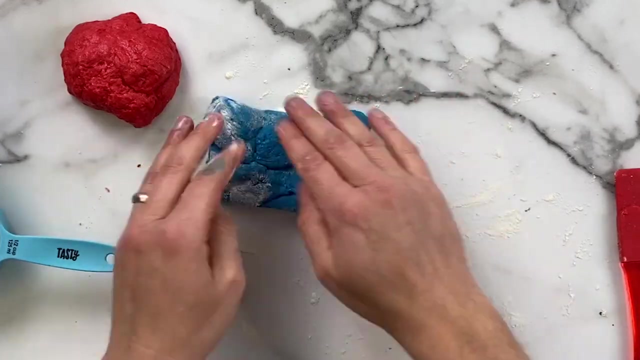 our red. Here we go with our blue. Look, There's barely any really come laying onto the table, Which is a good thing. Add a little bit more Flour. Pick up that color. I just dropped This. it just smushes so easily, So cool. 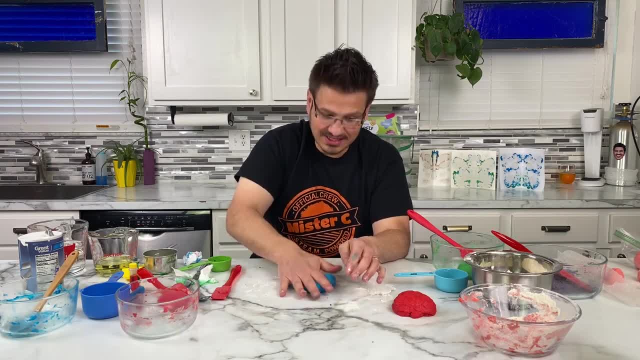 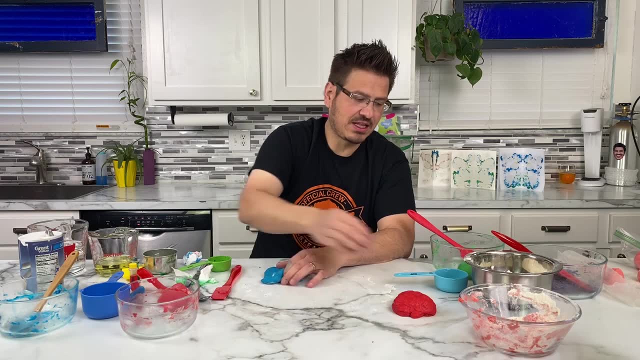 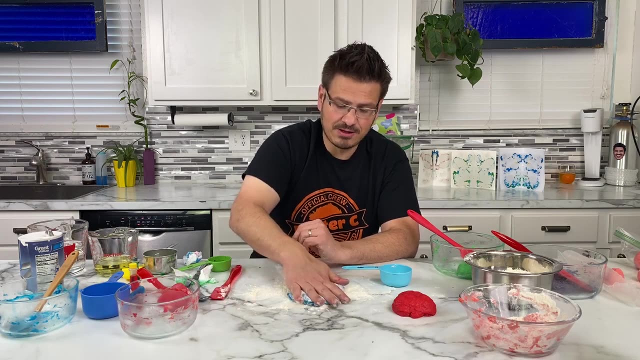 All right. so for sensory activities, this is really amazing. this is really amazing. I definitely like that a little bit drier, so I like it with a little bit more flour. that's just a personal preference. it doesn't have to be that way, but this is an opportunity for you to try different recipes and get 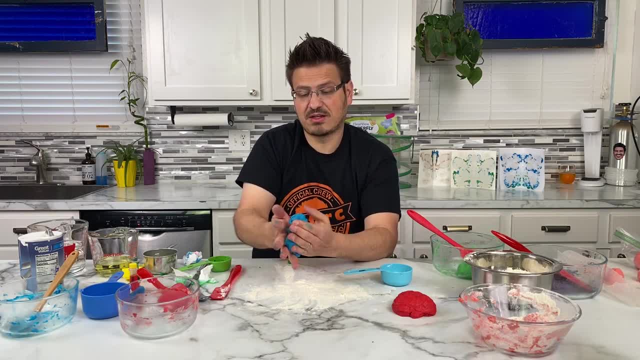 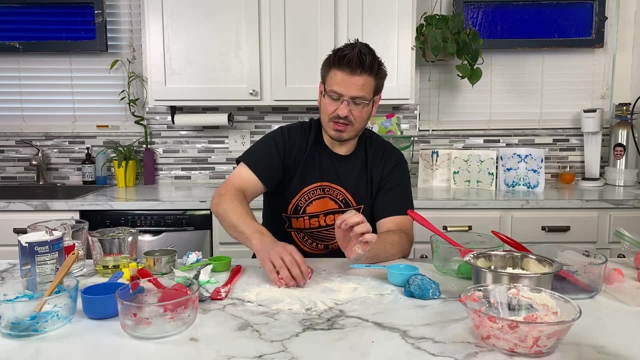 the one that you like, perfect, the one you like the most, perfect. all right, so we've got our blue. but I've noticed- did anybody notice? it's not holding a shape very well, so I'm just gonna- I can't really get it into a circle- I'm gonna. 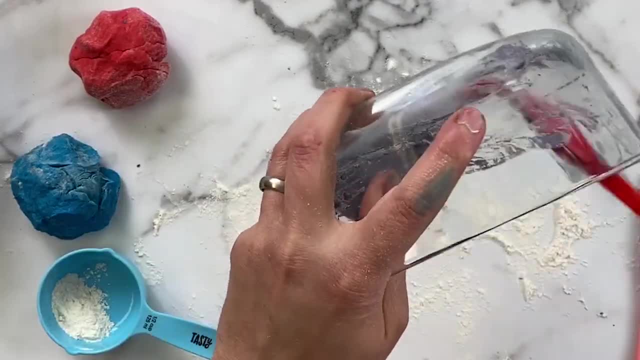 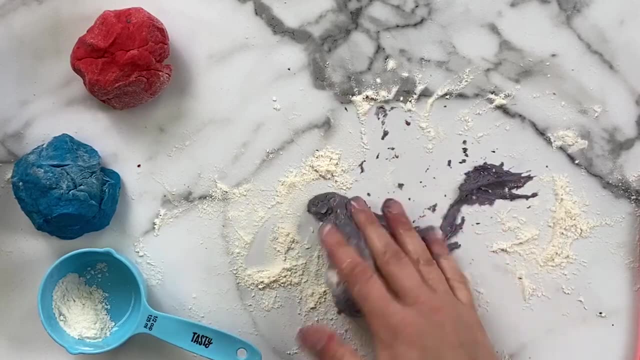 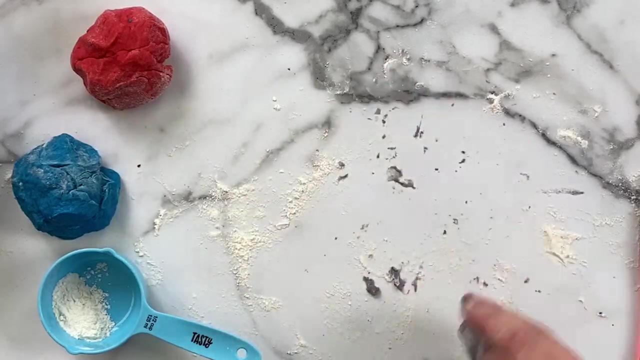 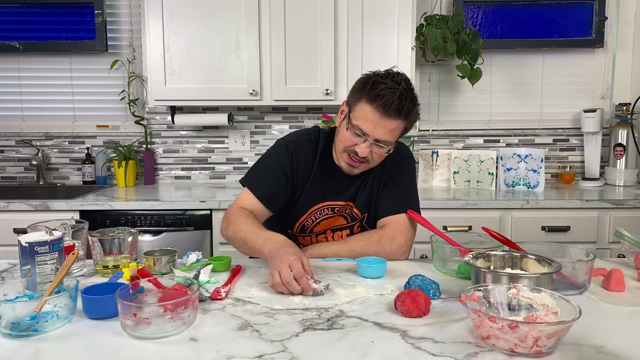 set that there. we'll see what it looks like here in a second. all right, here's our purple. we already got some. oh, that's so gross looking. definitely need more flour on this one. it's sticking on everything. oh, I got some other colors mixing in. I've got it really done. 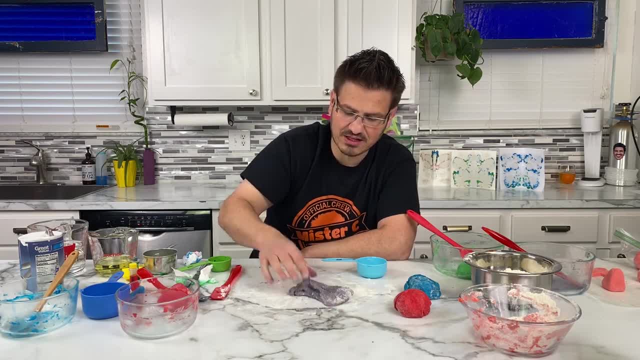 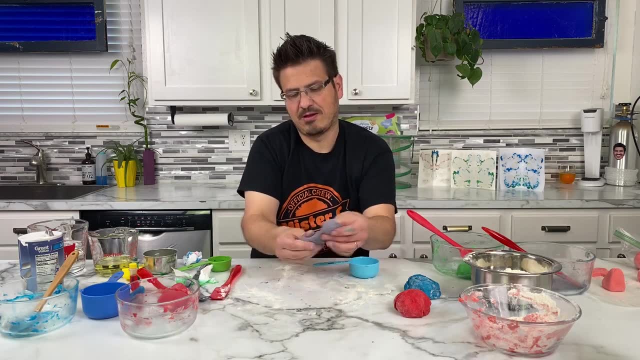 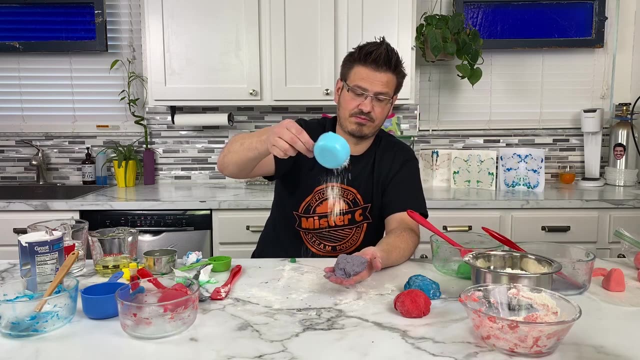 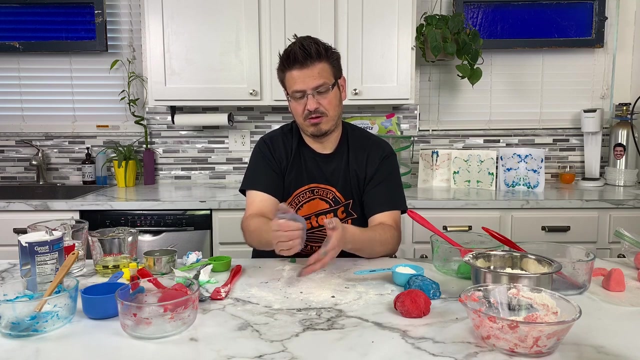 okay. so I'm gonna go ahead and take a look at our gray patch, and that's because of the flour, so that I think this color is gonna be interesting. what it looks like, it's sticky. oh, this one's really sticky. I thought I measured everything the same. maybe I didn't. 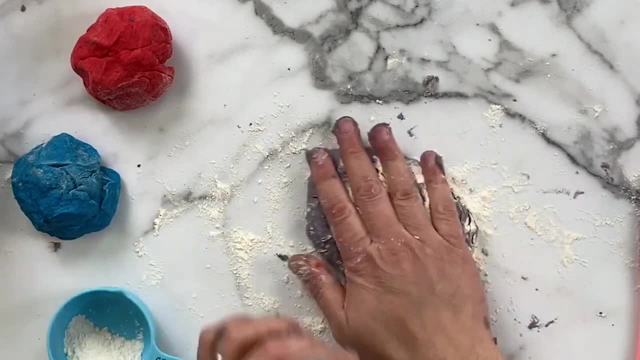 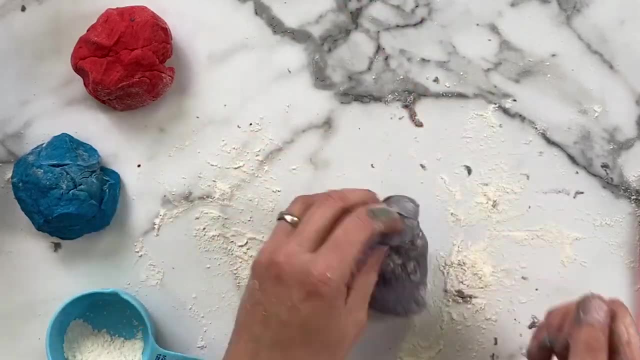 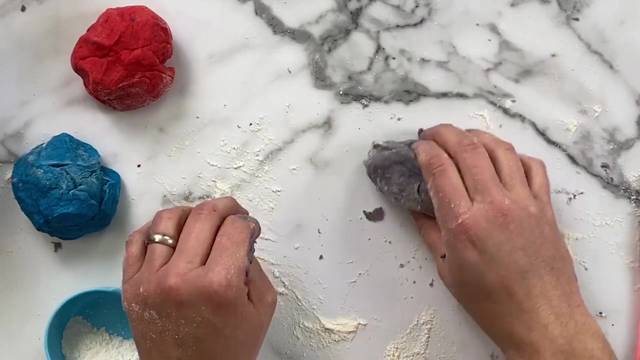 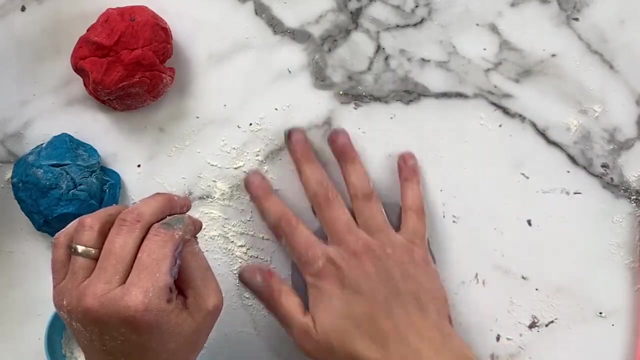 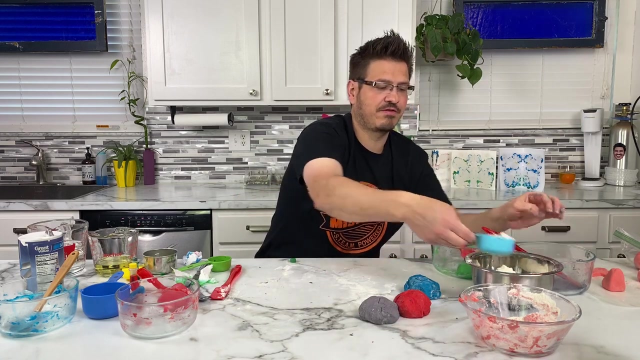 all right, it's still really sticky there. we go all right, so that's pretty good. on the purple slash gray: so yeah, you can lighten up your color by adding more flour as well. all right, and then we have our last one. I'm gonna throw a little bit of powder on first. this is what I'm. 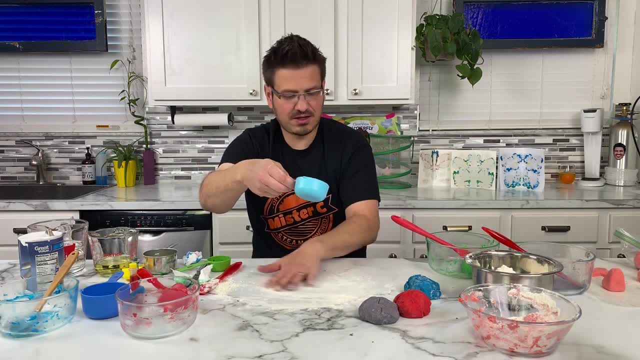 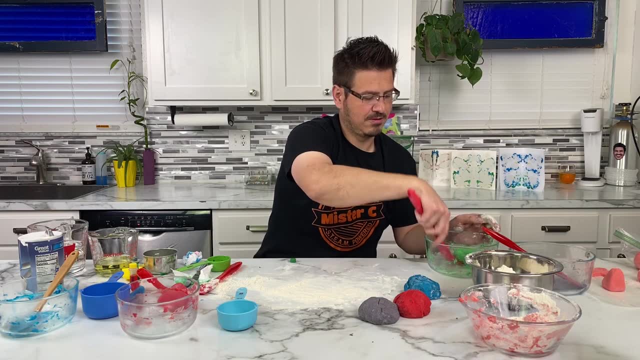 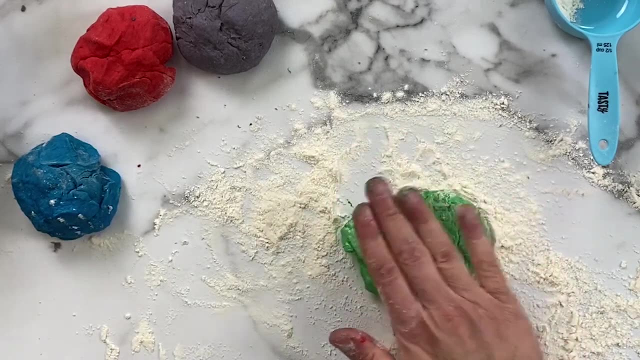 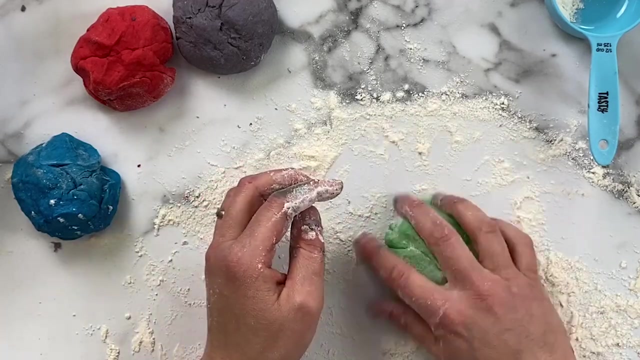 trying to avoid. I don't want to get these little chunks of other colors in, but it's okay. but my green and it's all over my hands, that's the real. I think that's where I'm getting more of my clumps from. so there you have it, we've 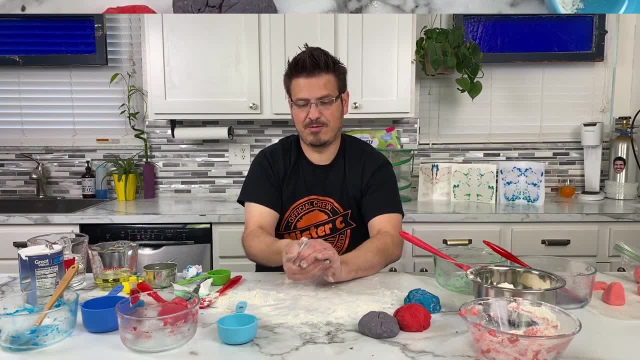 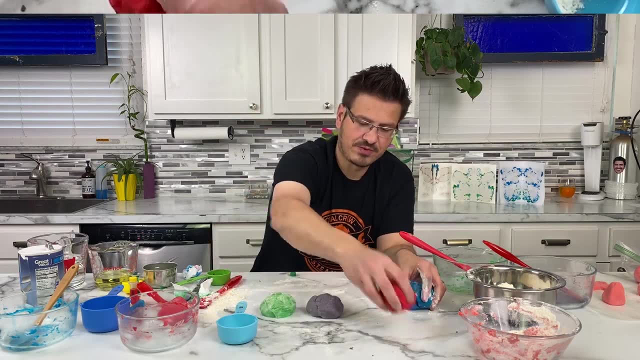 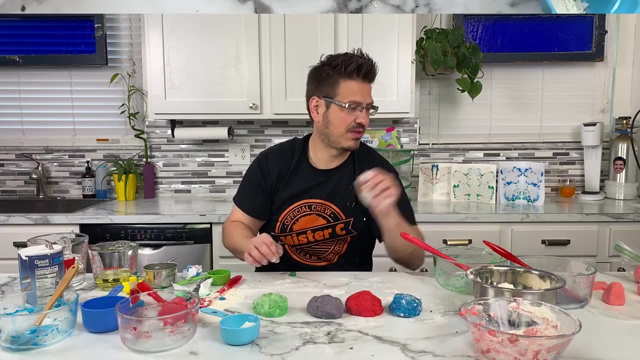 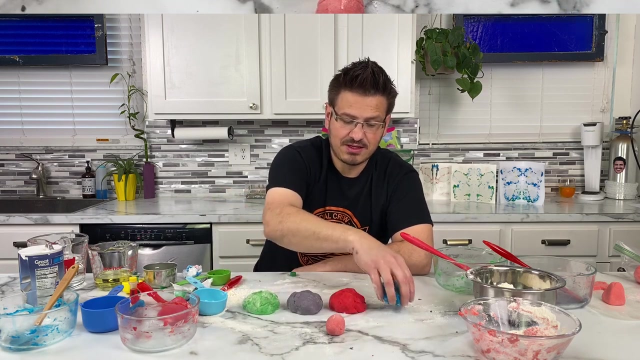 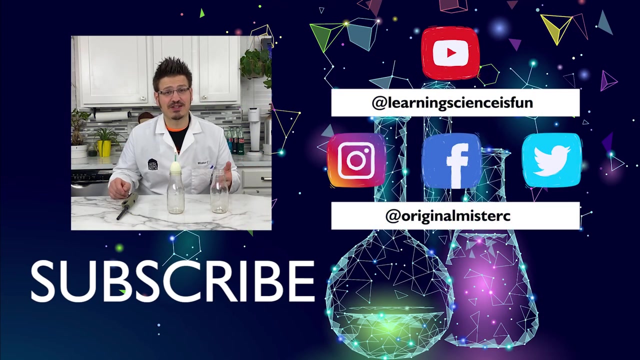 got green, purple, red and blue. now these obviously are not holding. these are not holding the shape the same way as our salt is, but the texture of these are just amazing. they really are. if you like that activity and want to see more egg experiments, make sure you like and subscribe to my channel and I'll see you in the next video. see you soon.